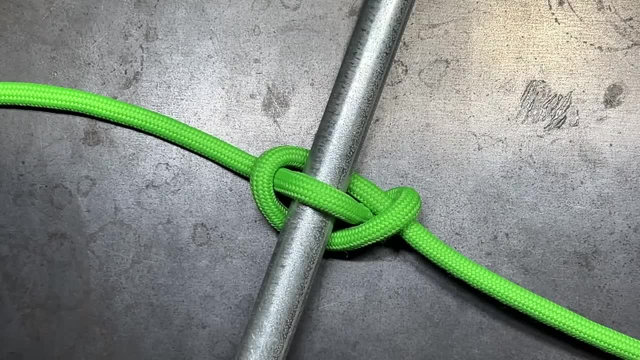 hitches. So hopefully this video will help you to get a little bit more proficient, and a lot of these knots are going to be the building blocks for a lot more complicated knots. So with that, let's get started Now. one of the easiest knots to learn is the simple overhand knot, The 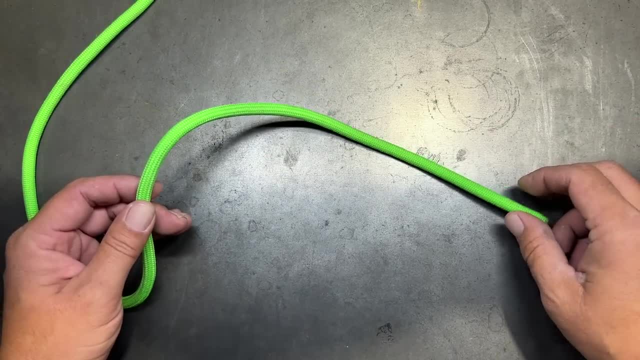 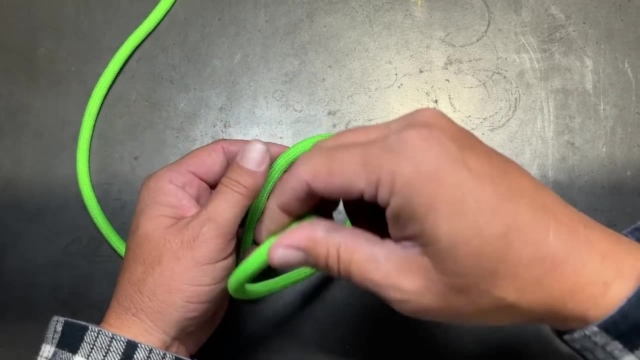 overhand knot can be used as a simple stopper knot or as a basis for a lot of other different knots as well. So to tie the overhand knot, what I want to do is we're going to just create a loop and then take your tag end around the standing end and then bring it back up through that loop, and that is the. 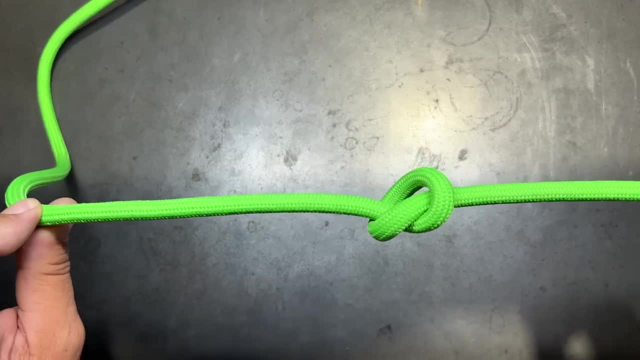 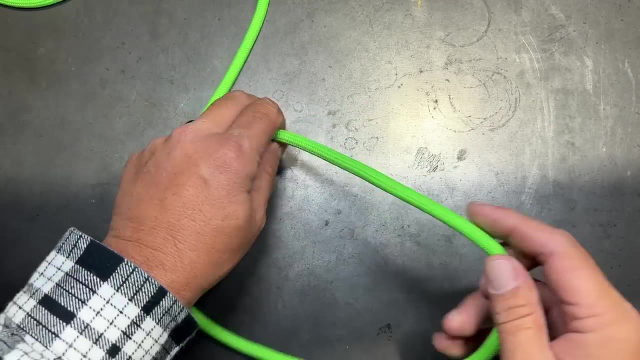 simple overhand knot. Now the overhand knot again can be used as a stopper or a basis for a lot of other knots as well. Now, if you know the overhand knot, it's pretty easy to turn this into a fixed loop knot too. So to do: 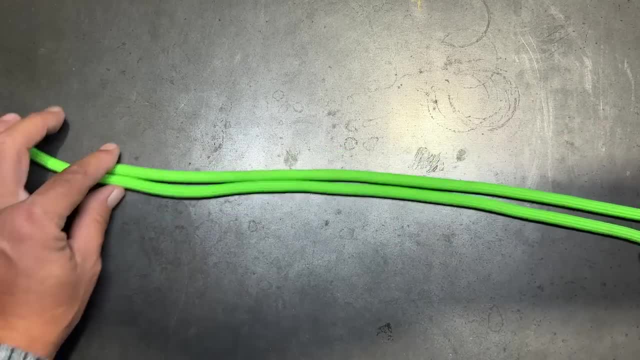 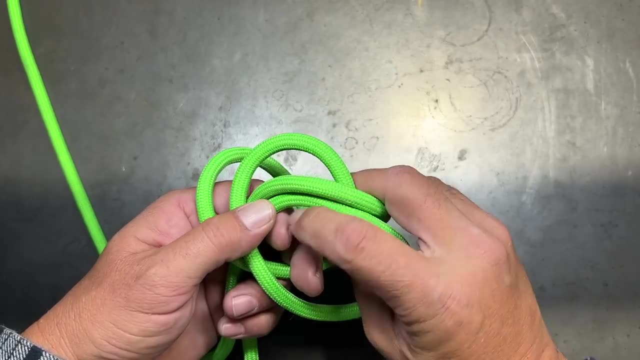 that what we want to do. instead of using just the end of the rope, we're going to double it over into a bite and then we're going to, with the two lines, we're going to form the same motion, go around back up through the loop, and that is going to create a simple fixed loop knot using the overhand knot. 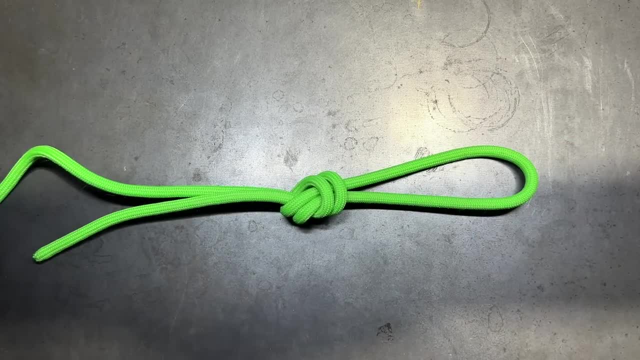 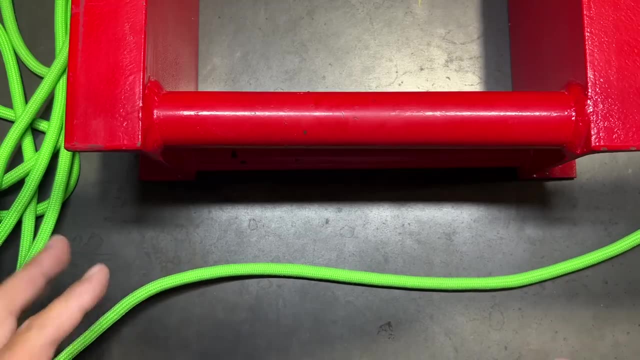 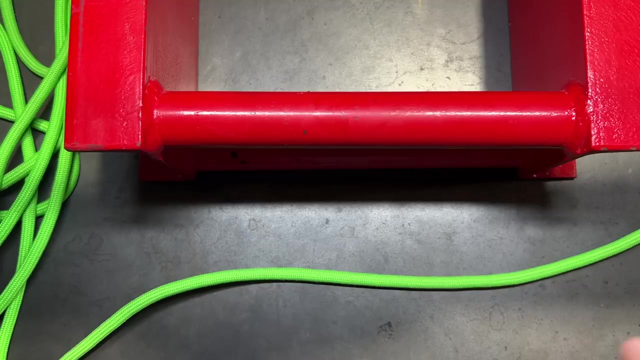 So this is a very important knot to learn, primarily because it's the building block for a lot of other knots. The next knot that we're going to look at is the half hitch. Now, the half hitch is generally used to lock off or tie off different knots so that they won't unravel on you. So the half hitch is a 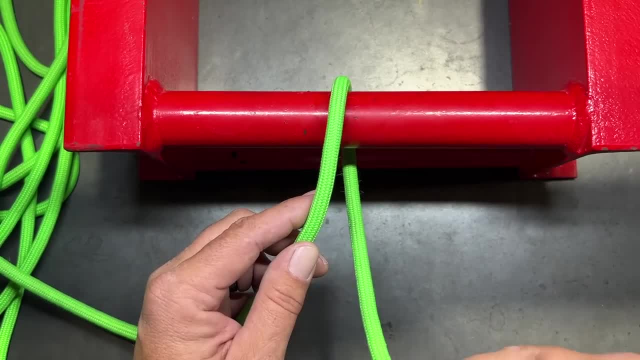 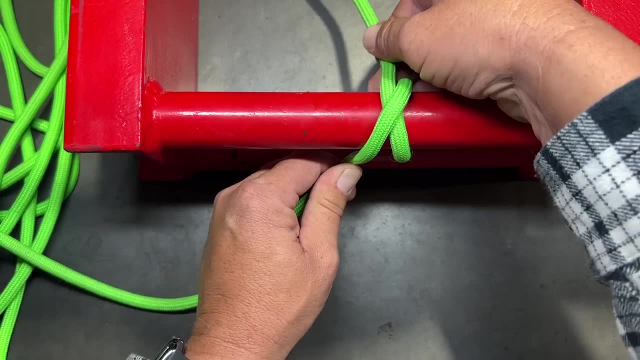 really simple knot to do. To do this, we're going to go around our object and all we do is tuck the back end or tuck the working end underneath the standing end. So the standing end will have pressure and the overhand knot is going to go around the overhand knot and then we're going to 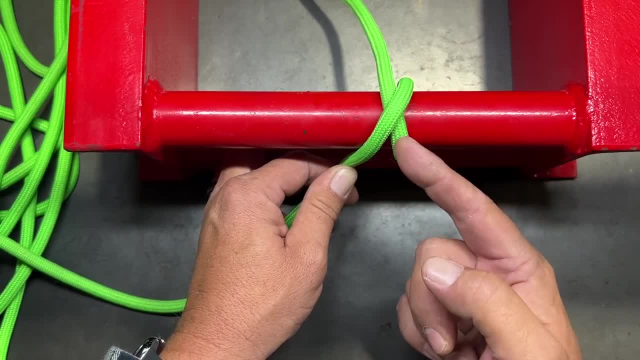 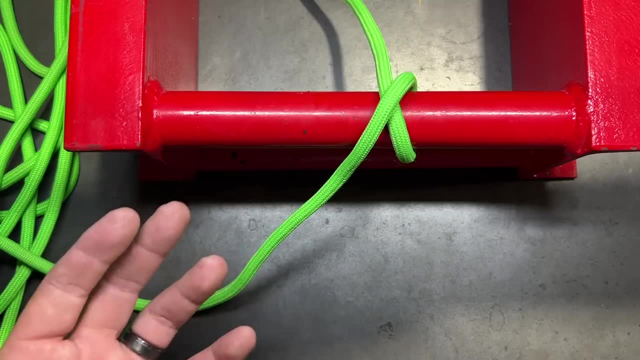 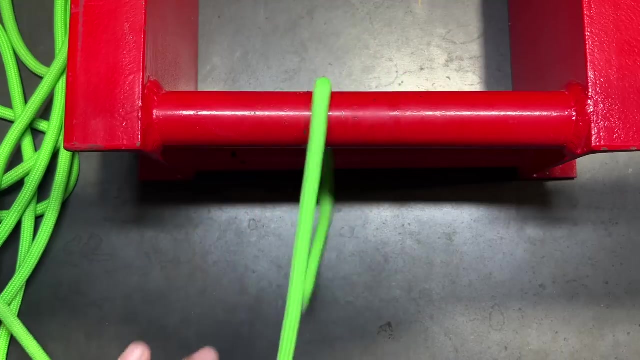 tie the overhand knot around the center, and what it's designed to do is to lock the tail end or the working end in place so that it will not come unraveled Now by itself. this knot is not used for anything in particular, especially for handling any kind of loads, because it very easily comes. 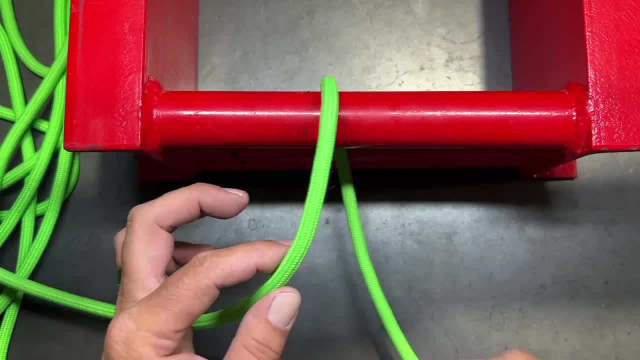 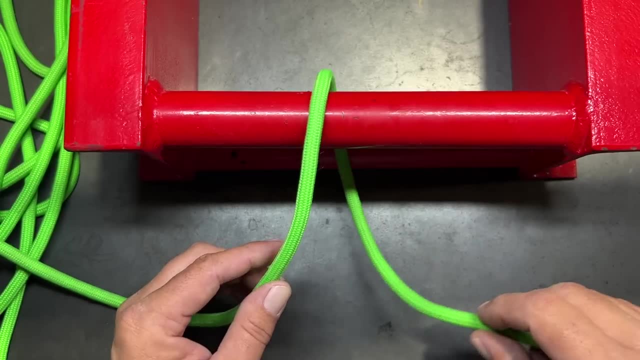 apart. Now there's another way to tie the half hitch and basically it's the same way that you would do the overhand, except this time we're going to tie the overhand around an object as opposed to itself, So we'll go around our object and then we'll go around the back side of our standing end. 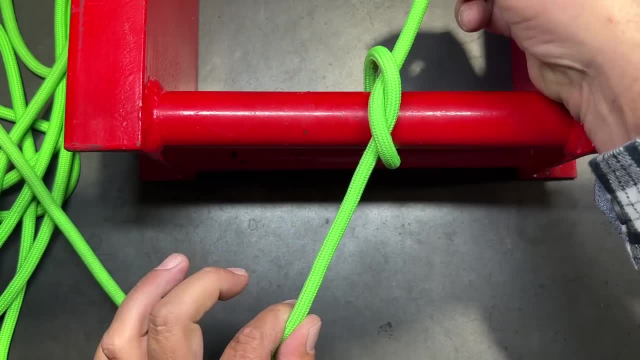 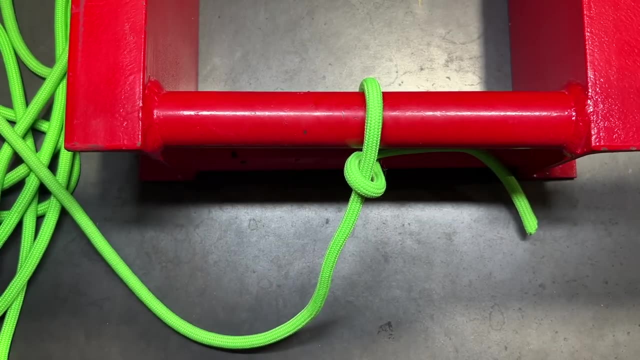 come back through the loop and instead of pulling it up like this, you'll pull it down, and this is also a half hitch. So there's a couple of different ways to form it. It's not very useful by itself, but it is incredibly useful when used in combination with other knots. Now the next knot. 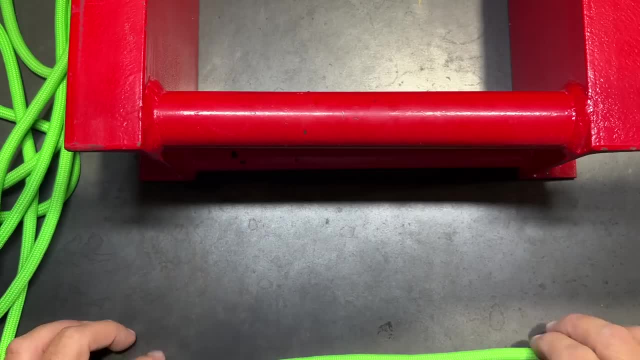 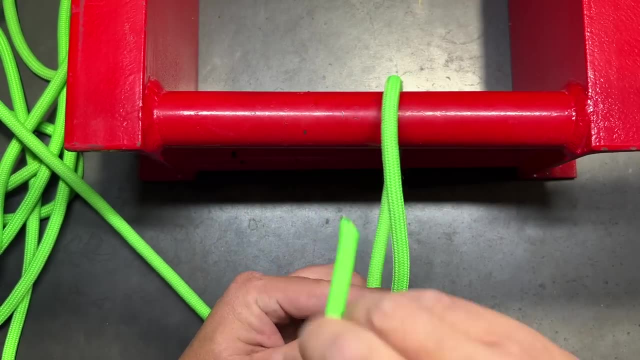 that we're going to look at is called the two half hitches. So, as the name implies it's going to be, we'll go around our object and, much like we did the half hitch down here at the bottom, like so we want to create the half hitch around the standing end of our rope and I'm going to give myself just. 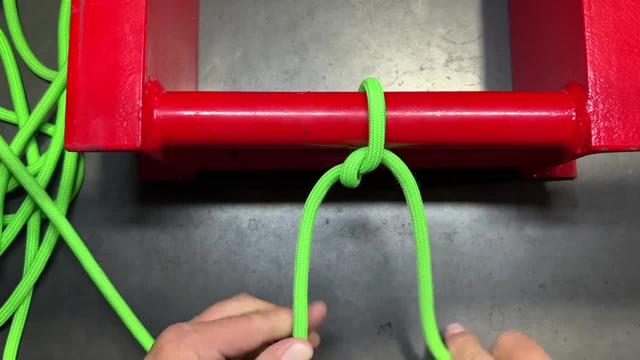 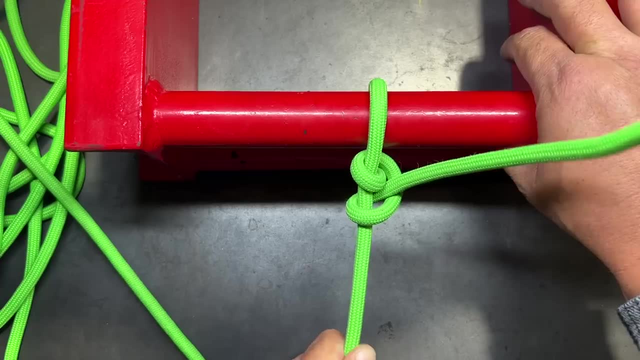 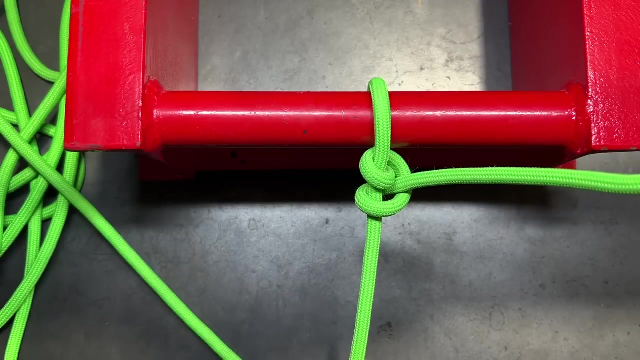 a little bit more tail in there. So we'll tie that first one and then we'll just do that process one more time, and this is the two half hitches. Now, the two half hitches is kind of a light duty application, so if you want to tie up a rope to an elevated position, this is a good, quick knot to learn. but 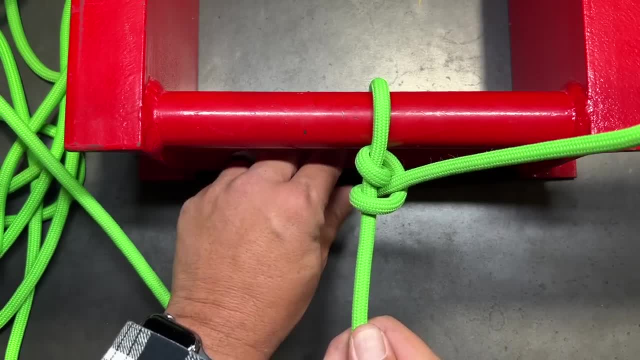 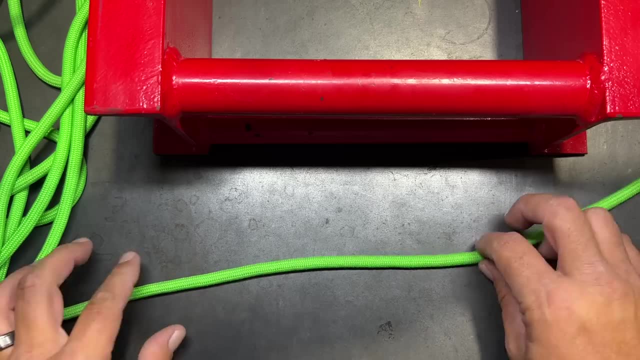 if you want to tie up a rope to an elevated position, this is a good quick knot to learn, but when you're doing a lot of these tricks you need to have a few knots. that would be better if you have a critical load that you need to hold. The next knot that we're going to look at. 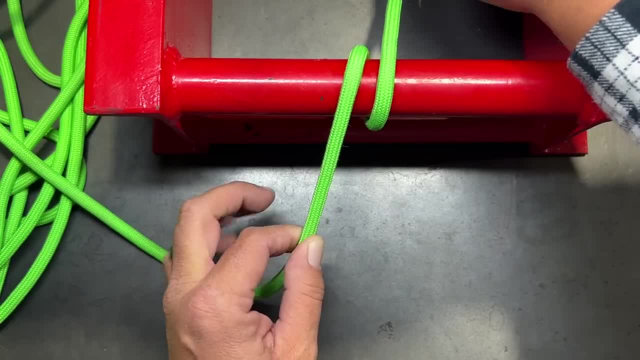 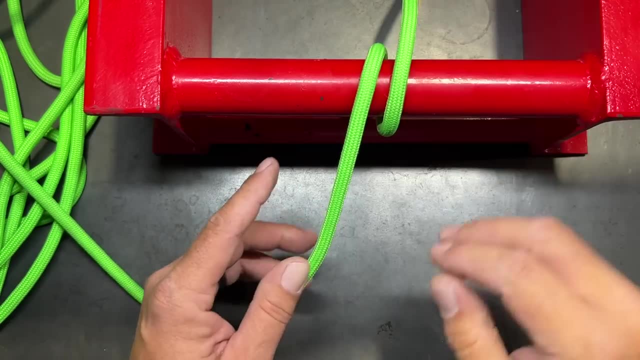 is called the round turn and two half hitches, and to do this we want to go around our object first. Now, if we went around the object and we stopped in this position, that's actually a full turn, but that leaves the working end and the standing end facing in opposite directions. So we want to 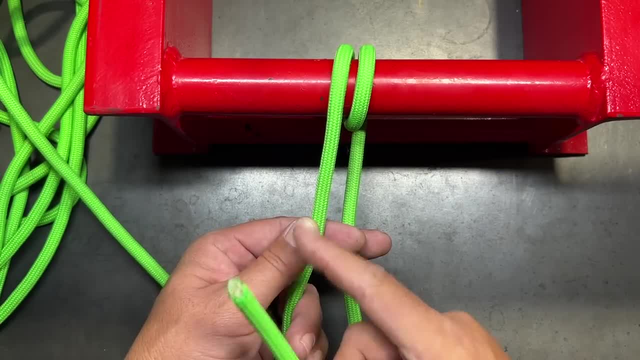 create a full round turn. The round turn gives us 540 degrees and 3.5 degrees- And we're going to do this with a half hitch in the bottom of the boot- and then puts the working end and the standing end in the same on the coming out the same side. 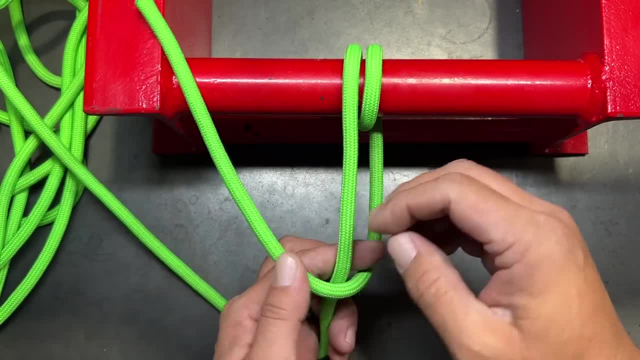 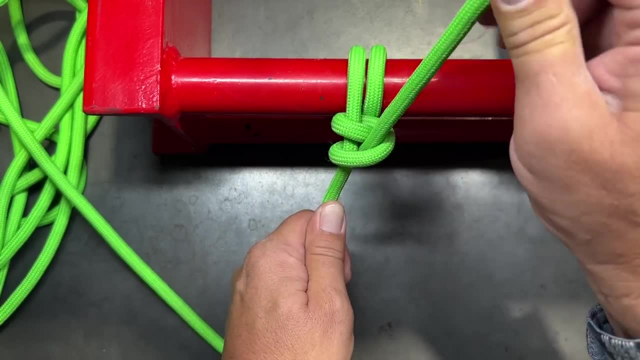 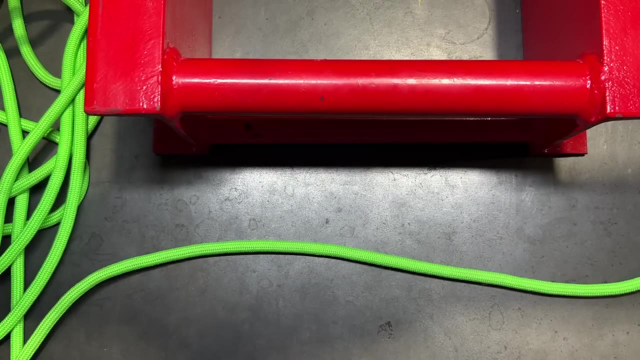 and so that is the round turn. Now, as the name implies, we just want to create two half hitches. so we'll go one half hitch, draw it up tight, and we'll create another half hitch around our standing end. pull it up tight, and that is the round turn. and two half hitches. The next knot is a very 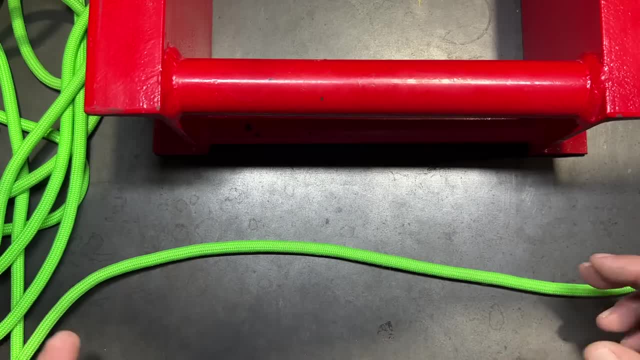 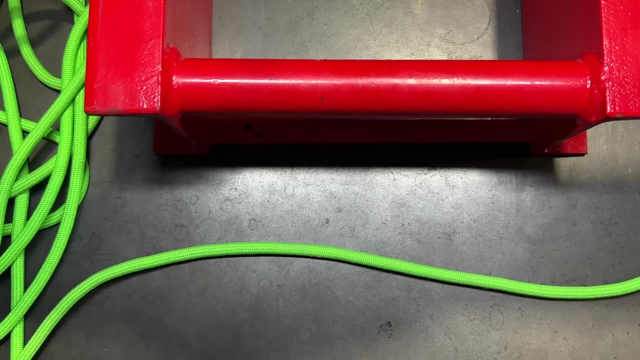 important knot to learn because it's a basis for a lot of knots. Now, this is a knot that I don't generally trust by itself, but is very important to learn in order to use it in other knots as well. that's called the clove hitch. So to form the clove hitch, we want to start off by going around. 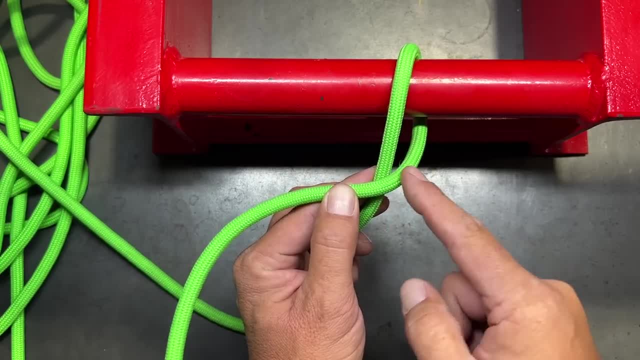 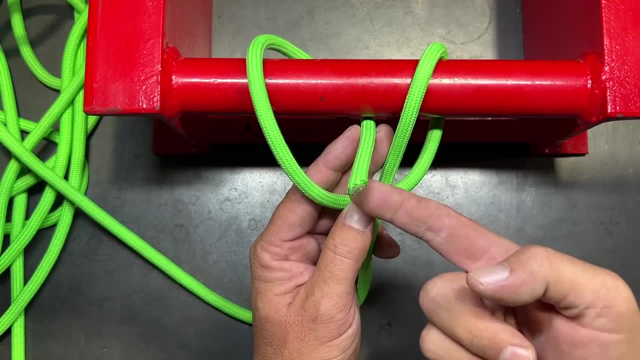 our object, then we're going to cross the standing end or, excuse me, the working end, over the standing end, and in the same direction, we're going to go around the object again, only this time, when we end, we're going to come up through this void that's left here, and then we'll pull the working. 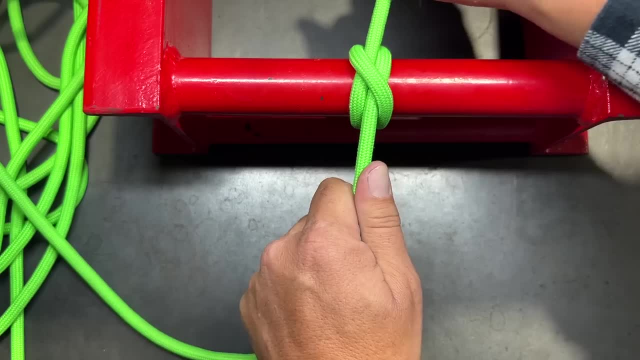 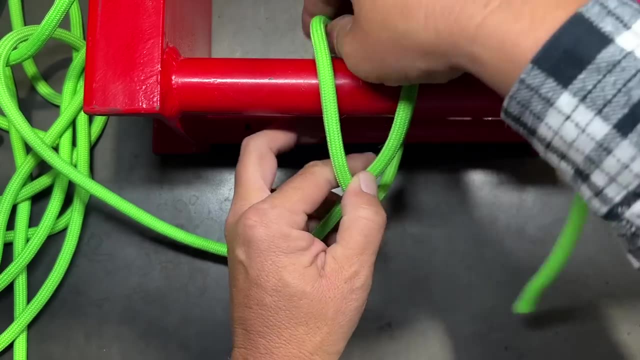 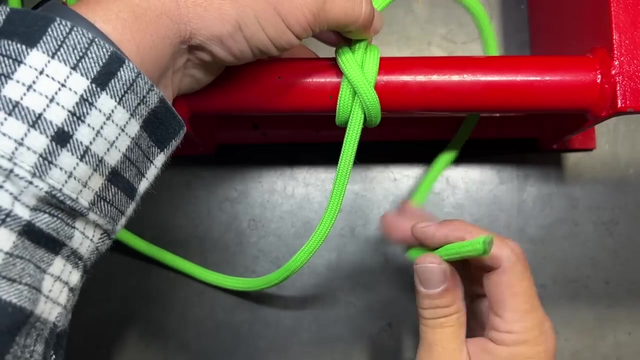 end and the standing end in opposite directions, and that forms the clove hitch. Now, as I mentioned before, the half hitch is a knot that's used to secure the ends of other knots. so here's our clove hitch and if we go ahead and continue the tag in around or the working in, 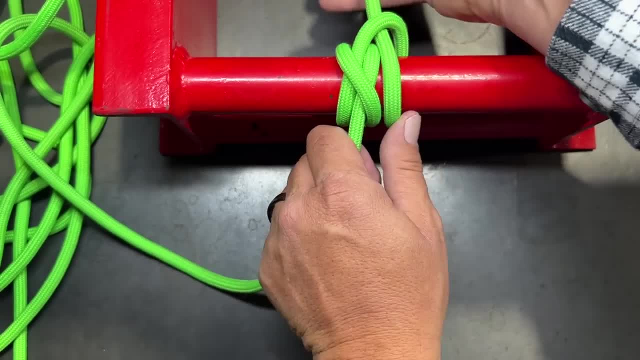 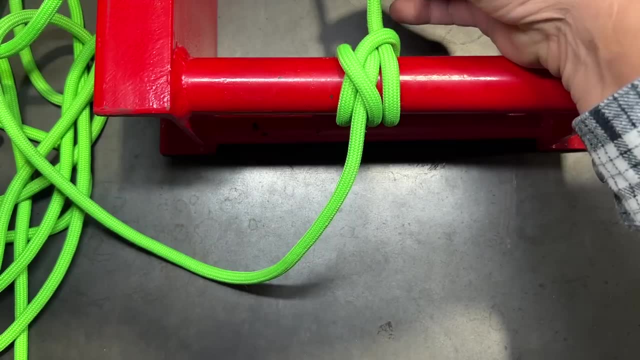 around and we create a half hitch at the end of this. this is a very popular knot. it gets used a lot. this is the clove hitch plus half hitch, and so you can see how the the clove hitch or, excuse me, the half hitch here at the end of the clove hitch actually works. 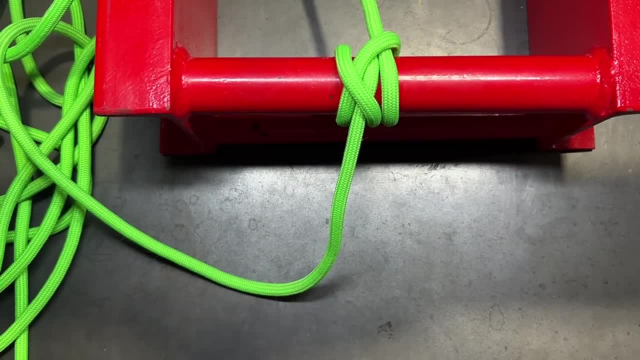 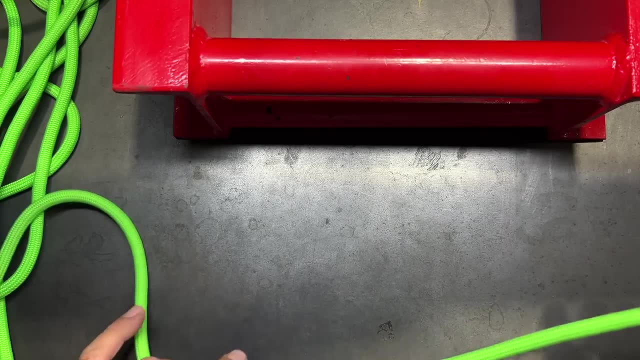 So this is a great way to keep this in place, so the clove hitch won't unravel. The next knot that we're going to be looking at is called the cow hitch. it's also known as the lark's head or the lark's foot. to form this knot, we want to start off by going around our object. 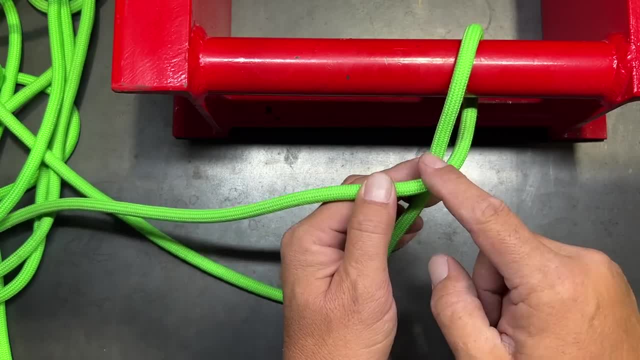 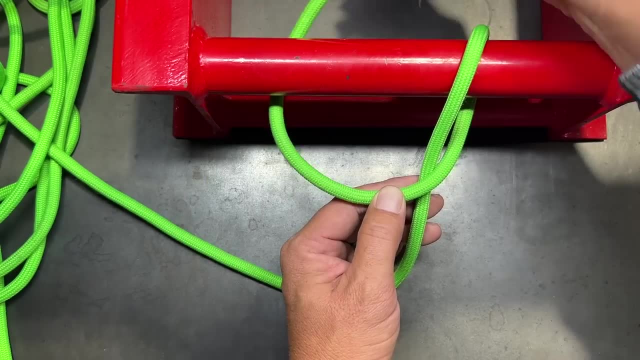 then we're going to cross over the working end, over our standing end, and this time, instead of like the clove hitch, where we would go over in the same direction, we want to change directions. we want to come up under and then send the working end back out the same direction or parallel to the clove hitch. 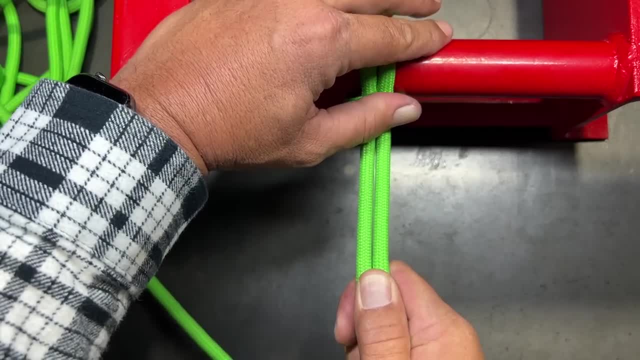 Okay. so now we want to work with our lark's foot to form our lark's foot. we're going to start off at the end of our standing end and then draw all that up tight and that is the cow hitch or the lark's head. 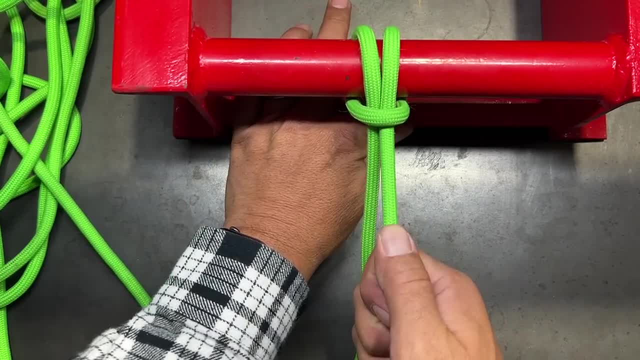 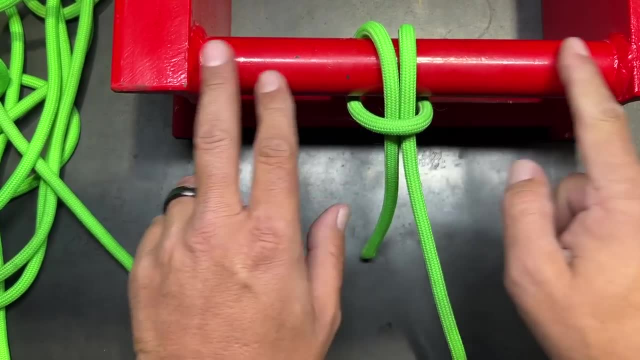 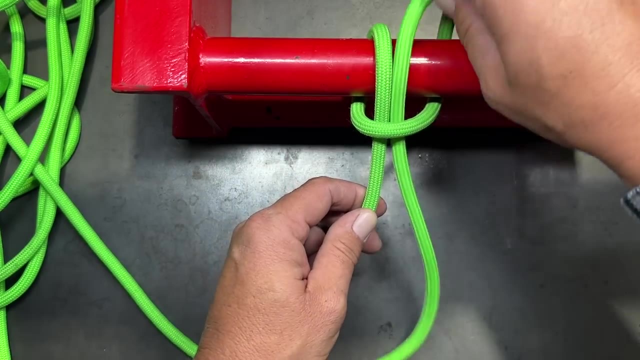 Now it's known as the cow hitch, because when you pull off, it's designed to be pulled off of just one end, but you can see that the cow hitch, especially on a slick surface like this, will tend to slip out. So you can improve this by doing what's known as the pedigree cow hitch. So we'll form our cow hitch and to finish it, what we're going to do is we're going to draw a line over the lark's foot with the t-shirt, and that will be the lark's head, And then I'm going to make a little bit of work on the top of the cow hitch and then I'm going to have to adjust that to the top of the lark's head. 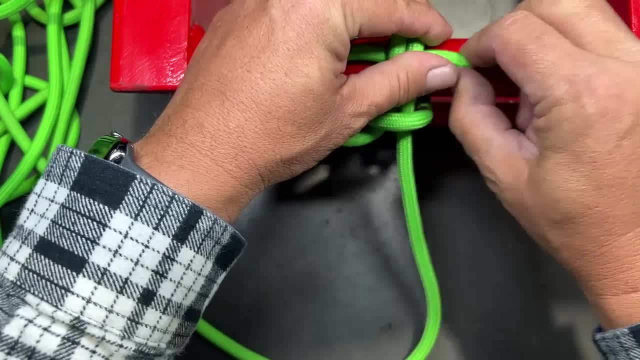 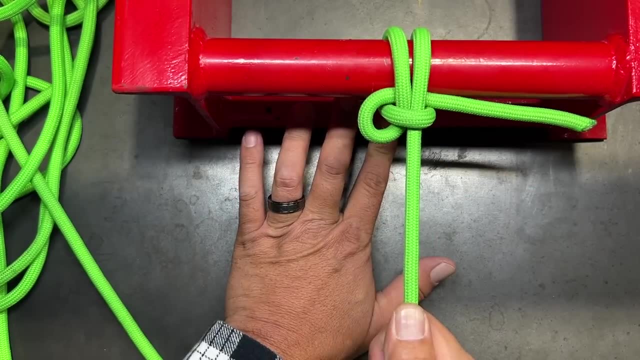 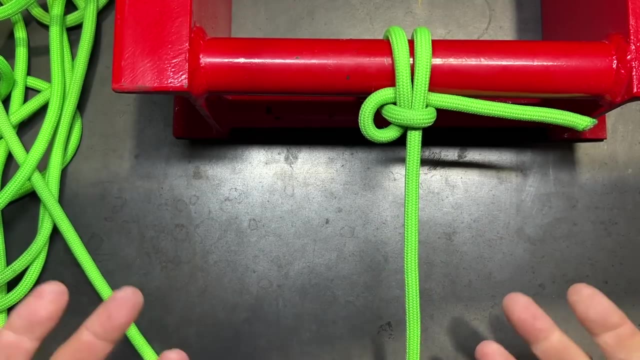 what we want to do is we want to lift up on our two lines here and then just tuck the end directly underneath of there, And that acts as a bit of a lock to hold the cow hitch in place better. Now it's known as the cow hitch because you're only putting stress or pressure on one. 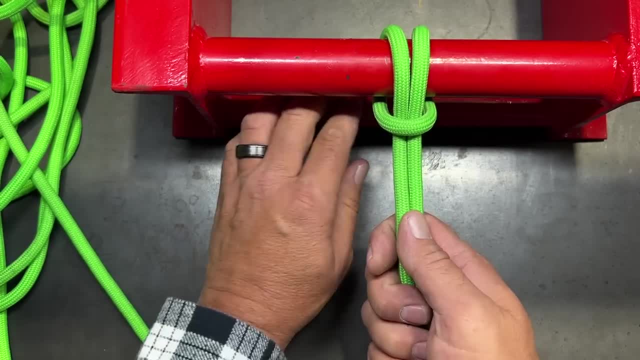 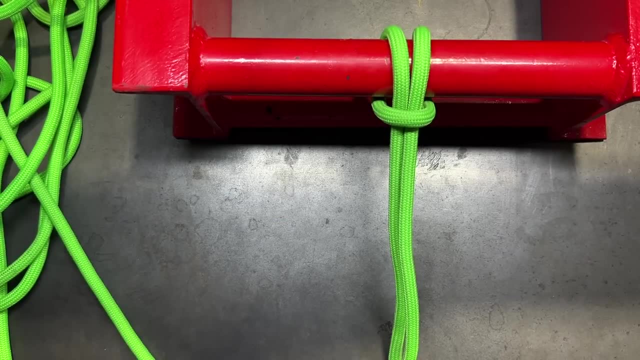 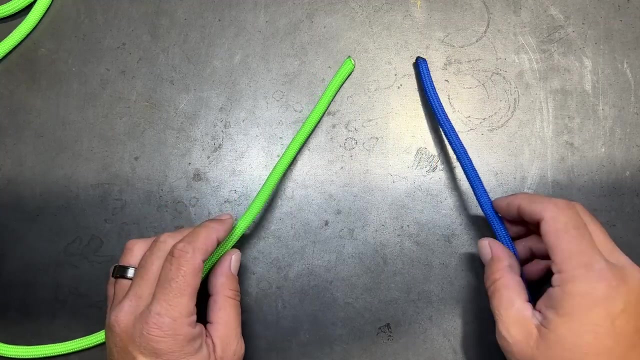 end. If you are putting stress on both lines, then that is called the girth hitch. So they're very similar, but it's the way they are loaded which distinguishes, which is which The next knot that we're going to look at is called the square knot or the reef knot, And this is not really a 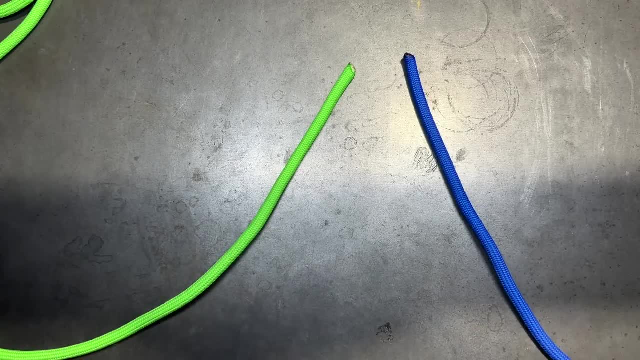 bend knot, where you would tie two lines together but more of a binding knot. So if you're tying together a bunch of books or a bunch of sticks, something of that nature, the reef knot or the square knot is a good option To tie this knot. we're going to take our two lines and first we're 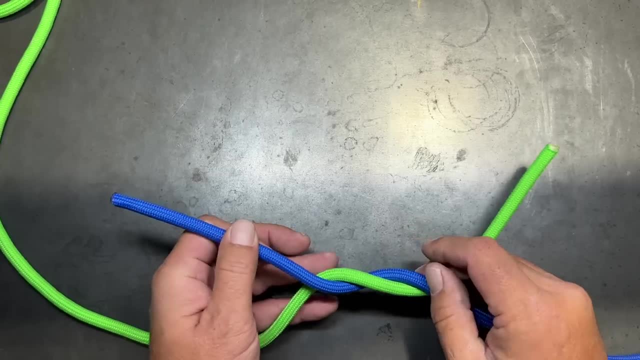 going to cross the right over the left, We'll bring it around, and then we're going to cross the left over the left, And then we're going to cross the right over the left, And then we're going to cross the left over the left, And then we're going to cross the left over the left, And then we're. 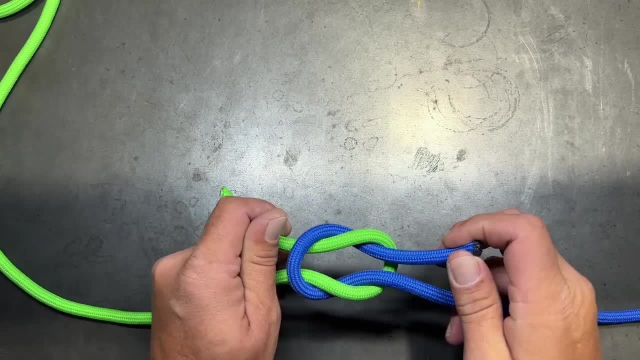 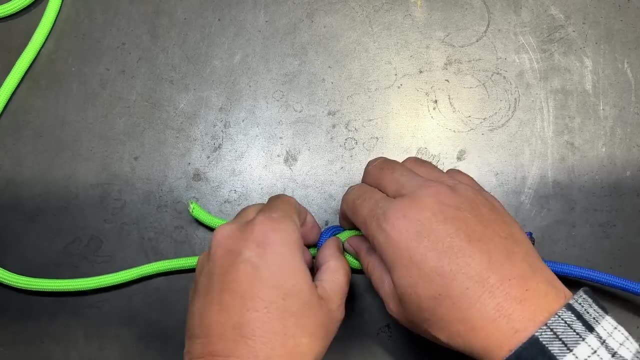 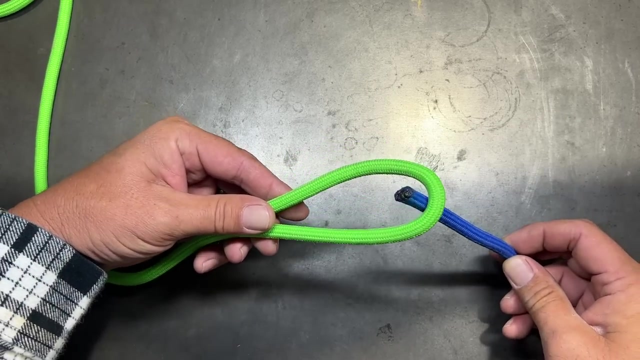 going to cross the left over the right and bring it around and then pull them apart. And that is the simple reef knot or the square knot. Now, it can be formed like that or it can. you can do it a different way. You can just form a bite in this line. Start by going up through your bite, then go. 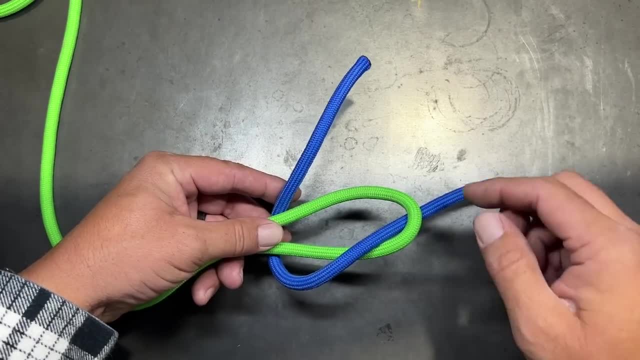 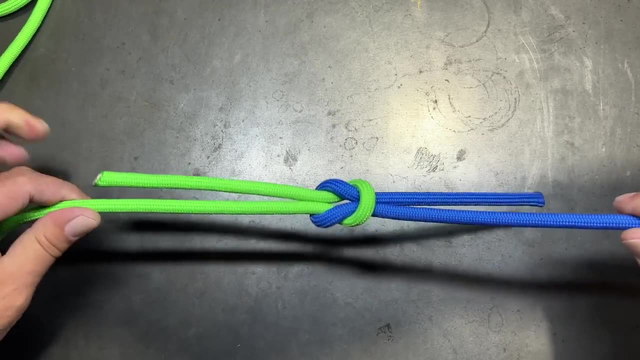 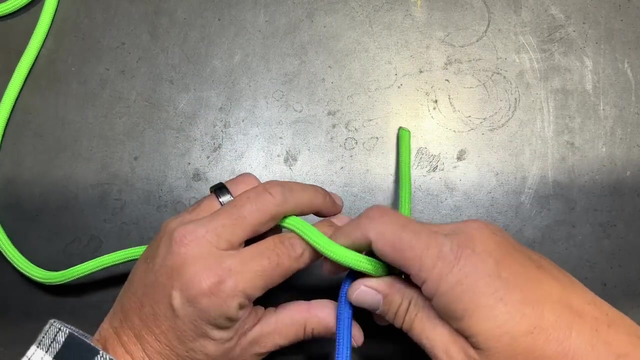 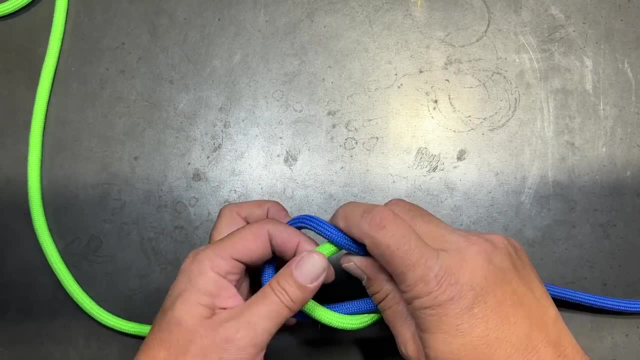 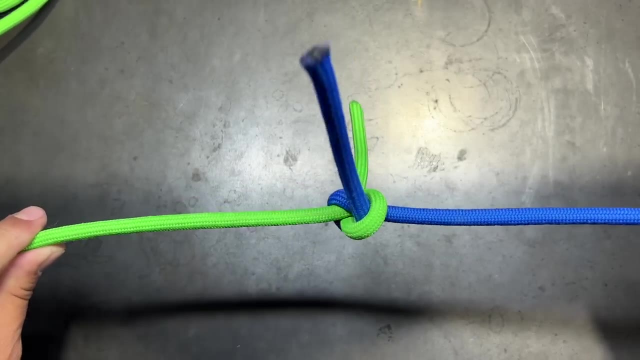 right on the next pass. if you go right over left again, what you end up with is a pretty inferior knot. This is called the grainy knot. So when we pull this apart you can kind of see this knot will actually give quite a bit, And it is definitely inferior to the square knot. The next: 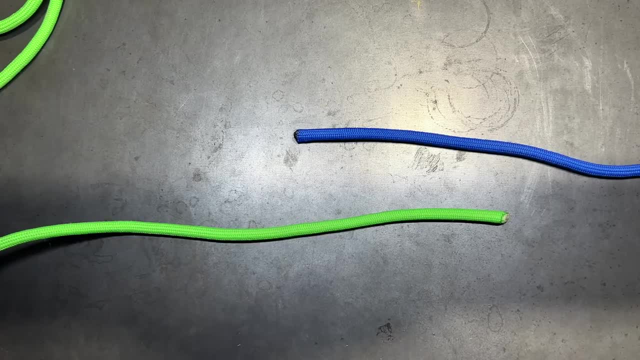 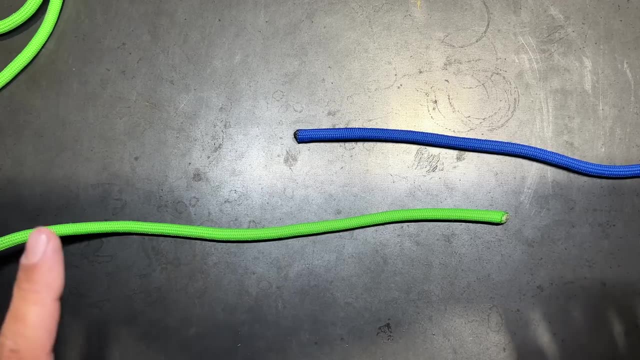 knot is the sheet bend, And the sheet bend is one of the most popular bend knots, though it's generally tied in its double form, And I'm going to show you that as well. So the sheet bend is used to tie two different ropes together. But you can. the benefit to this knot is that you can. 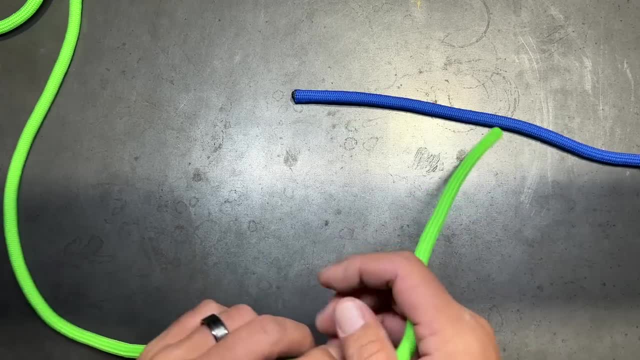 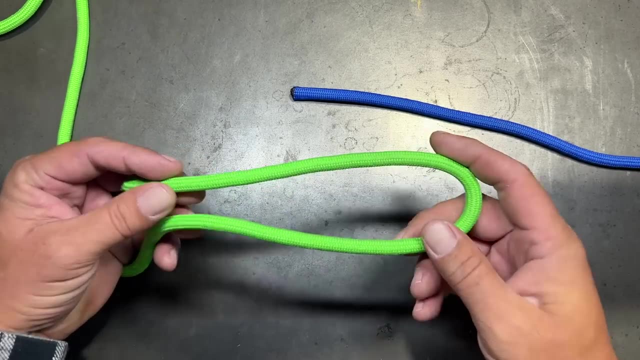 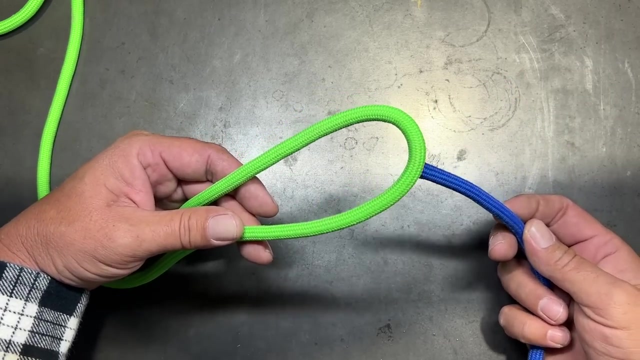 very easily tie ropes of different diameter together. So to start the sheet bend, what we want to do is create a bite And if you had two different size ropes, you want to create the bite in the larger line. Then we'll take our tag end or a working end from our other rope, send it up. 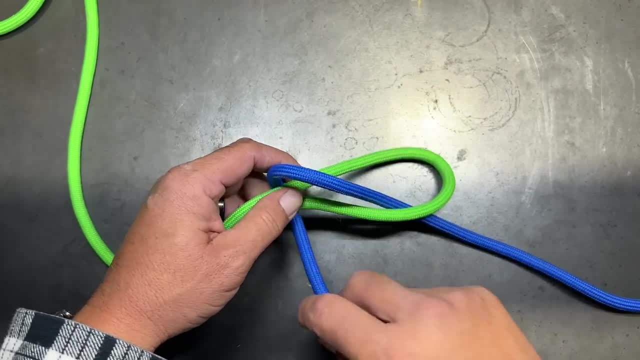 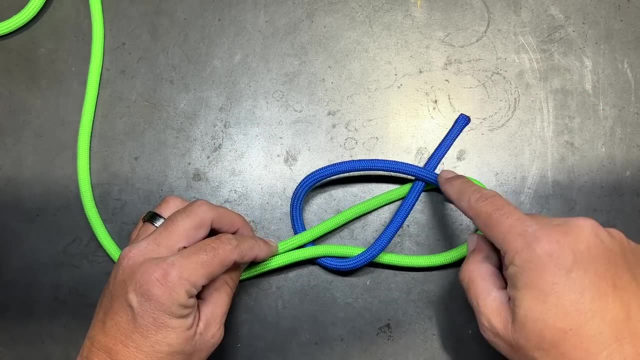 through the other end and then we'll tie it together, And then we'll tie it together And through there, and then we'll go around the backside and, unlike the square knot where we would just fall back in, We want to lift up here and we want to send the tag end underneath. 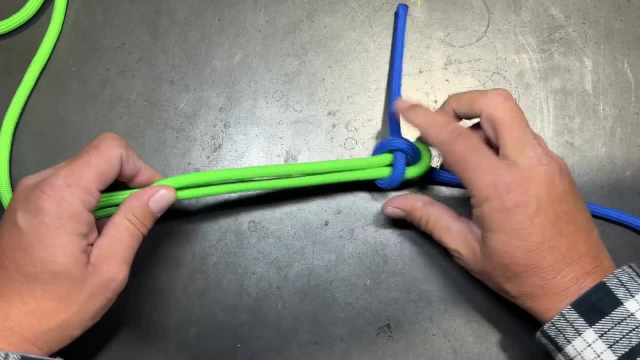 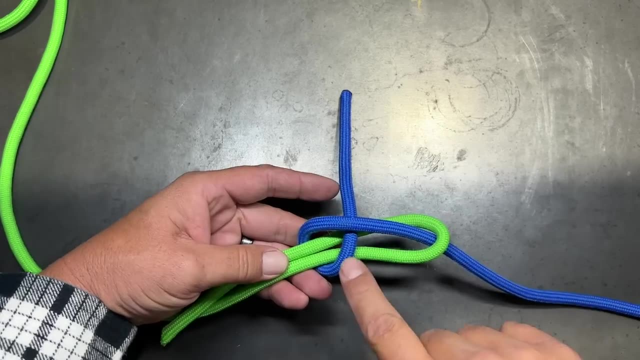 its own standing end and then pull them apart, dress your knot up And that creates the simple sheet bend. Now to form the double sheet bend. What you want to do is, instead of just ending here, You want to take one more wrap around and tuck it back. 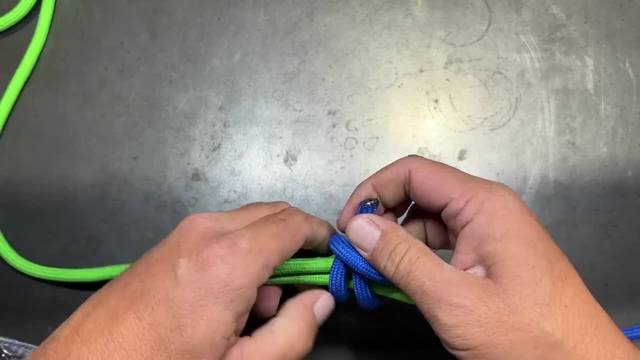 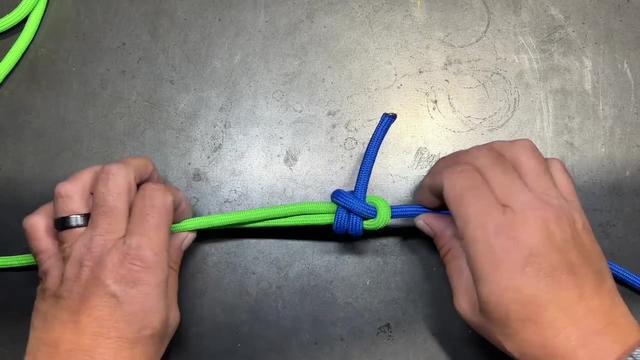 through And that creates the double sheet bend. You could also also turn this into a triple sheet bin or a quad sheet bin, whatever the situation requires, But usually this knot is tied in its double form, where you'll make two wraps that tuck. 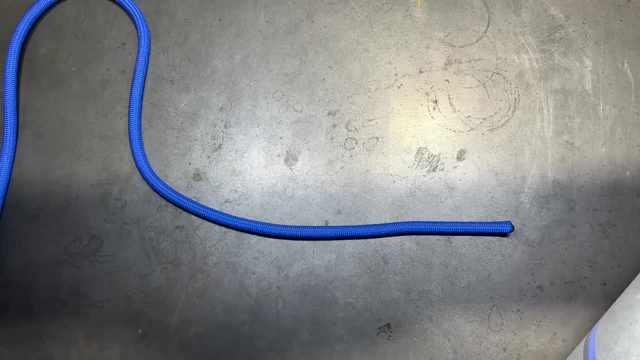 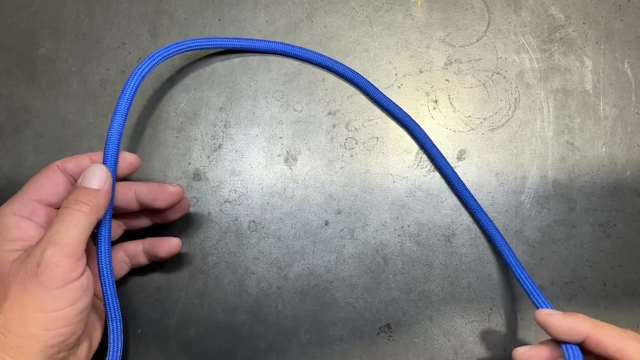 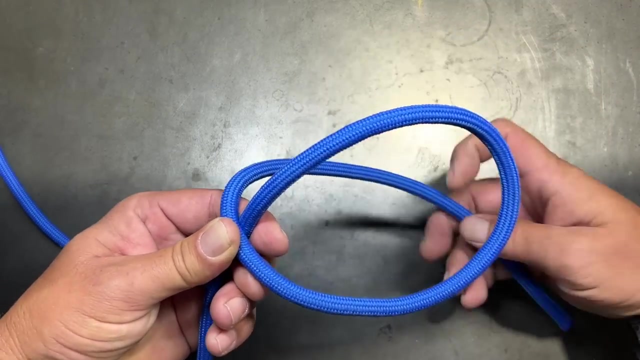 underneath of its own standing end. The next knot that we're going to look at is the figure eight knot. Now, the figure eight knot can be used as a stopper knot and is tied pretty similar to what the overhand knot was tied. So, to start this, we're going to form a loop and then, instead of coming up, 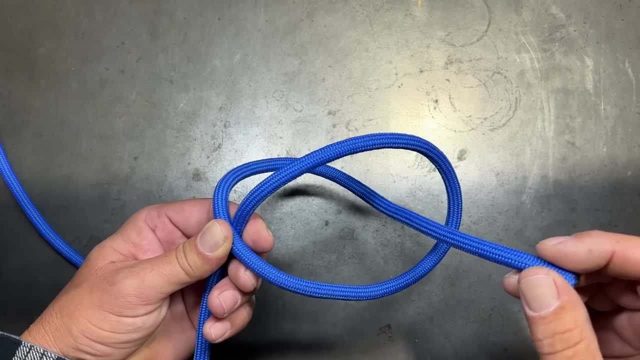 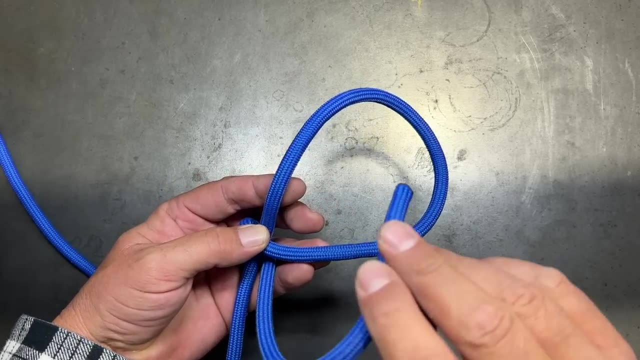 through the bottom, going around our standing end and coming up through that loop to form the overhand. we want to just continue around so that we go one full turn around the standing end and then send the working end through that loop in the opposite direction and pull. 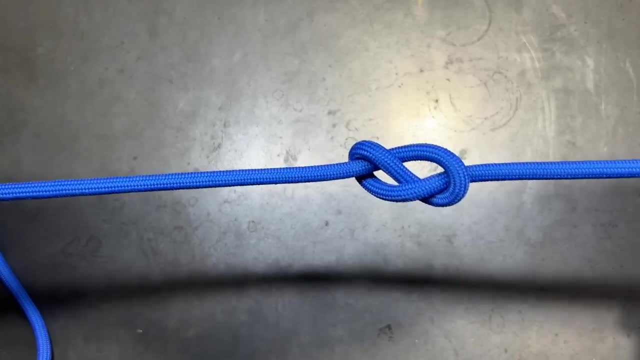 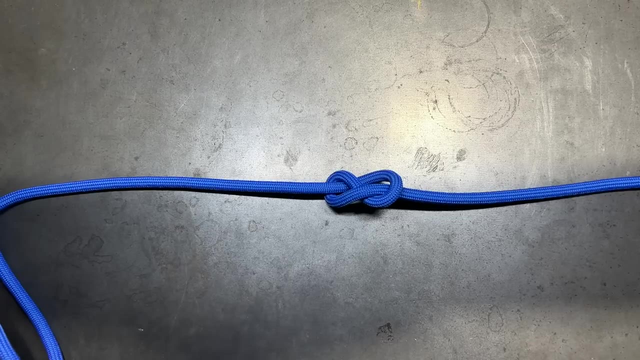 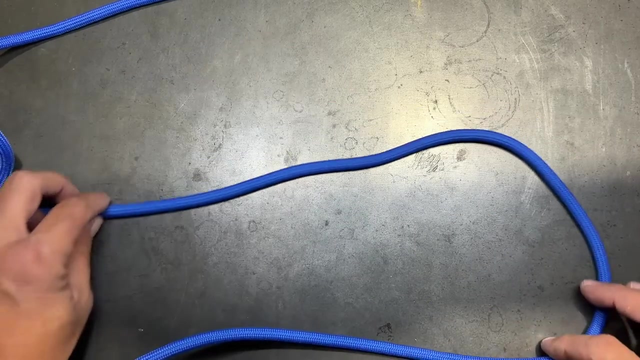 them apart. That forms the simple figure eight knot. This is a decent stopper knot, but it's generally used in climbing applications in a fixed loop. It's called the figure eight loop and it's very similar to tie. Uh, then, the same way that we tied the overhand to form it into its loop method. uh, the simple. 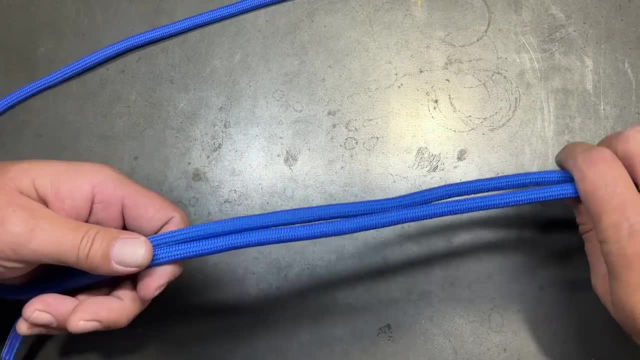 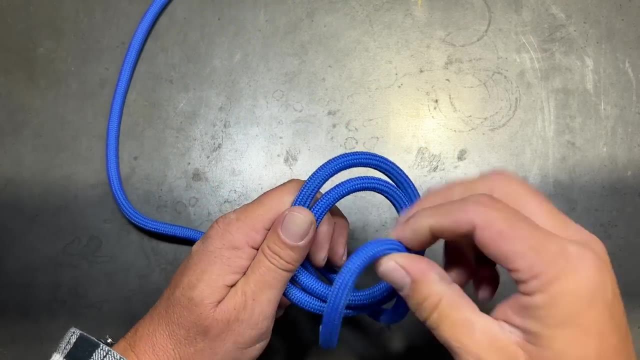 loop you want to take and form a bite, and then we're going to form this in exactly the same way. we formed the overhand by going around the standing end, one full revolution, and then coming back down through the loop there and then pull them apart and that forms the simple. 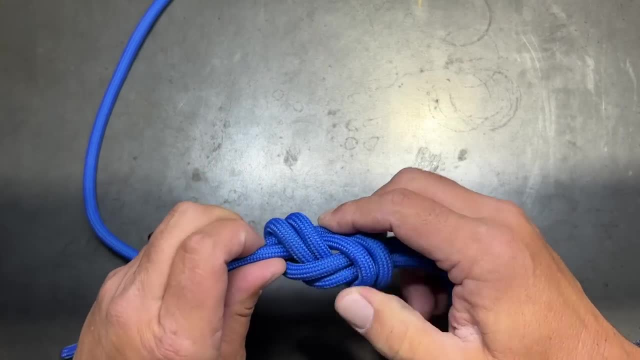 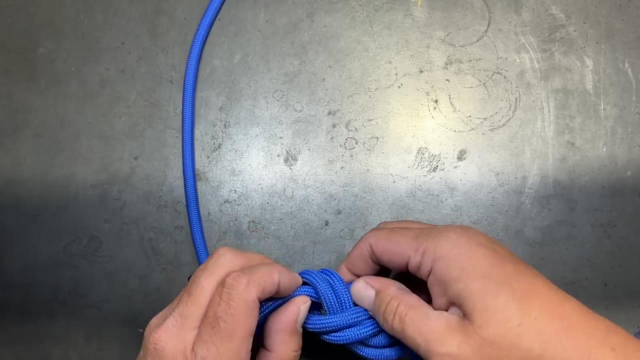 figure eight. Now it's important with this knot you just want to make sure that it all lays in there correctly, So you might have to adjust it. You might have to adjust the line so that you get all of your lines parallel, and mine's off a little bit here, So I'm going. 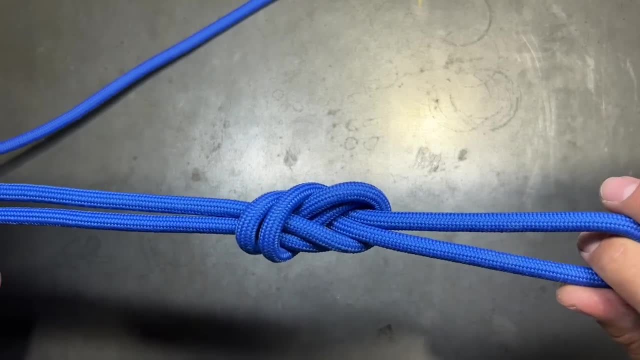 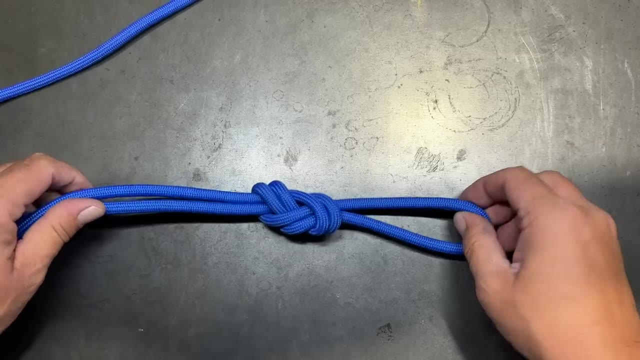 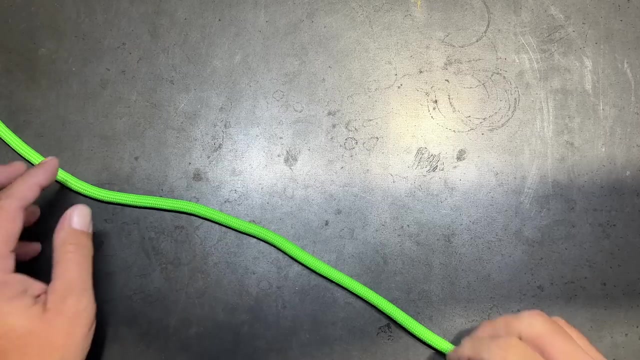 to adjust this just a little bit. The idea behind the figure eight is just to make sure that it lays in nice and flat, uh, to give you the best knot possible. So this is the figure eight loop based on the figure eight. The next knot that we're going to look at is the Marlin spike hitch, And this is a knot. 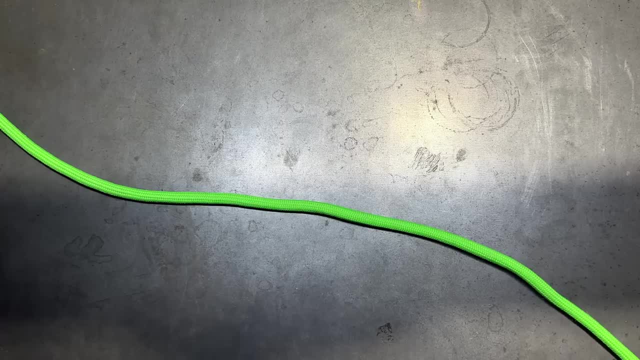 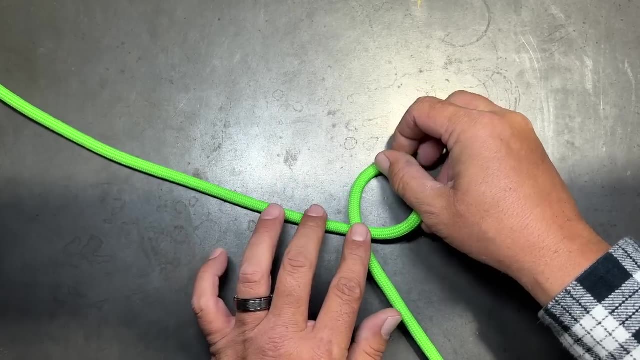 that I actually use quite a little bit. I use it more so for tensioning a line. So what we want to do Is: anywhere on our line, we want to lift, turn and create a loop. I'm right-handed, So I turn to the right. Now this is our standing end or, excuse me, our working end, And this: 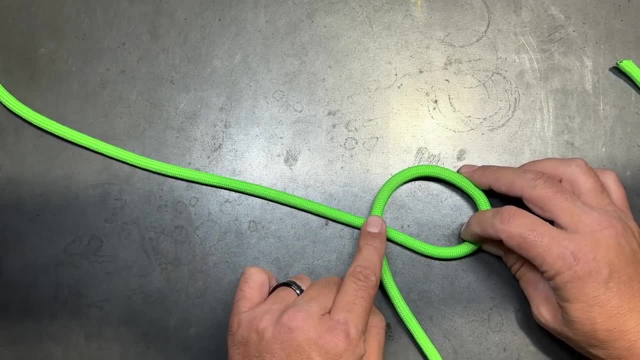 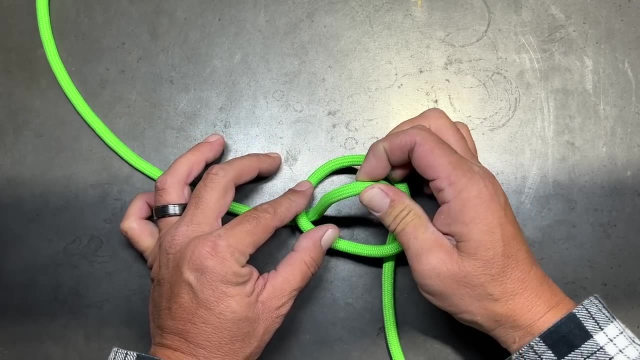 is our standing end. So we want to take this loop that we formed, kind of hold down the eggs and just bend that over the top of the standing end, like so. Then we'll pull a small bite of the standing end through that loop, And now all we have to do is set a toggle. 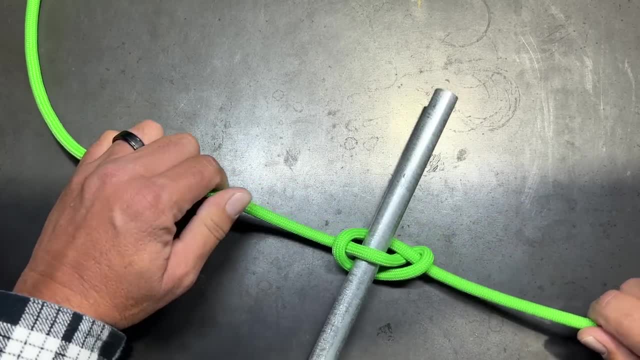 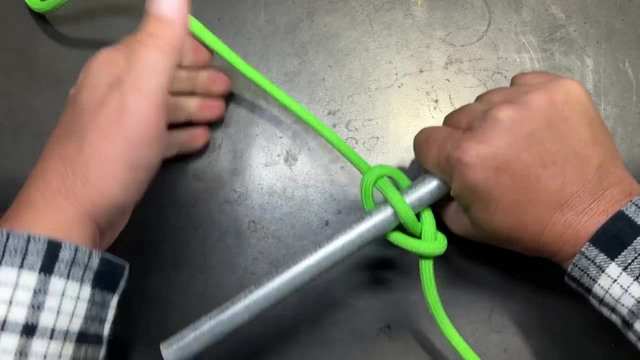 through there And now we can pull the working and the standing ends apart and that forms the Marlin spike hitch. Now this is used to pull tension against the standing end of the rope in the method that or the application that I use it for most. 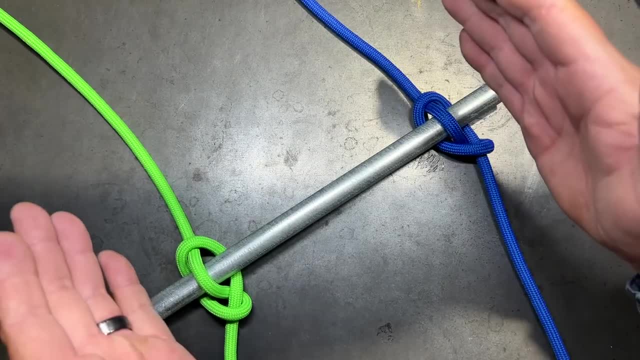 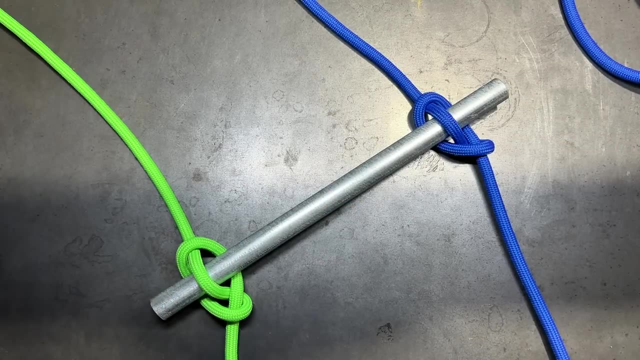 Now, another application that you can use the Marlin spike in is by setting two parallel lines with multiple Marlin spikes. Your toggle will generally be something like pieces of wood branch, where you would be able to create a makeshift ladder. So you can imagine if 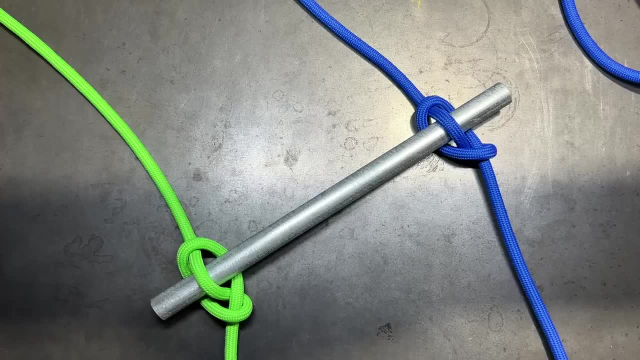 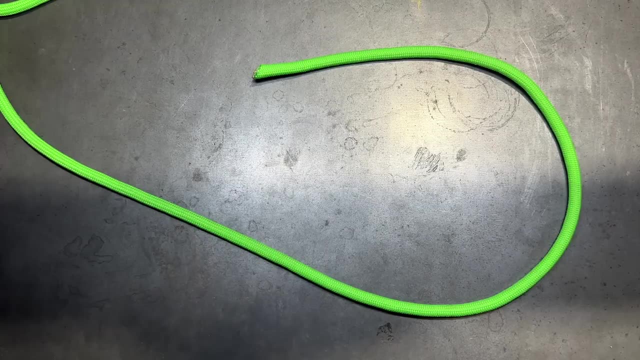 you add multiple Marlin spikes- Spikes you can evenly spaced- and you have a pretty sufficient ladder for emergency situations. The next knot that we're going to look at is called the bowling, and the bowling forms a fixed loop knot is one of the most important knots that you can learn. There are so many. 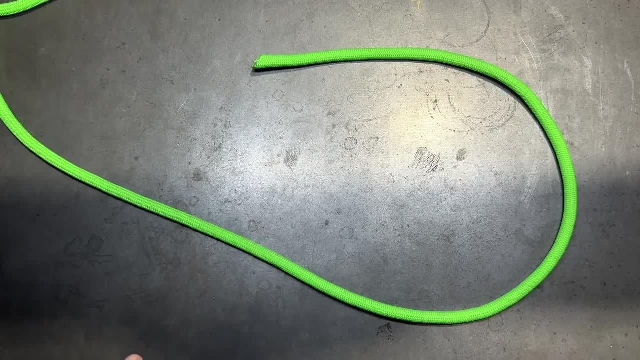 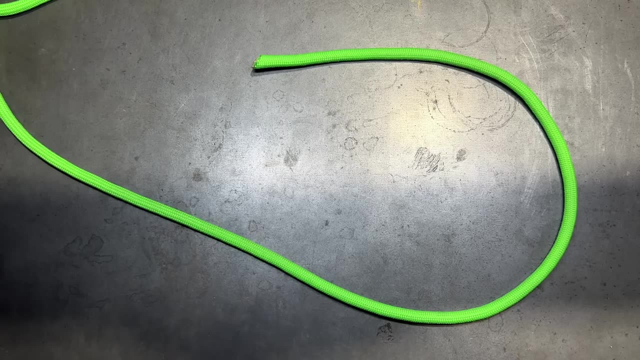 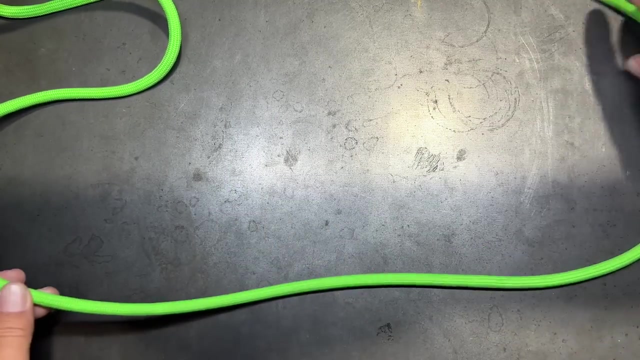 different applications for the bowling, and I actually have a video that shows multiple ways to tie this knot and the reason why I consider it the king of the knots. So, to tie the bowling, what we want to do is: you want to create a loop, So I'm going to go down about 18 to 24 inches down the rope, depending on. 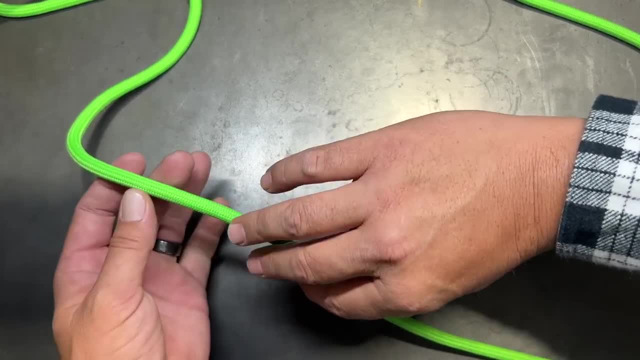 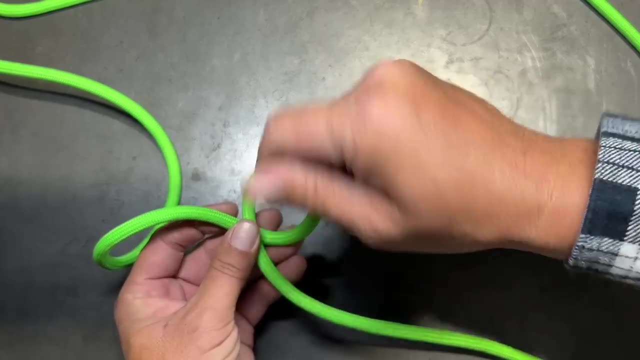 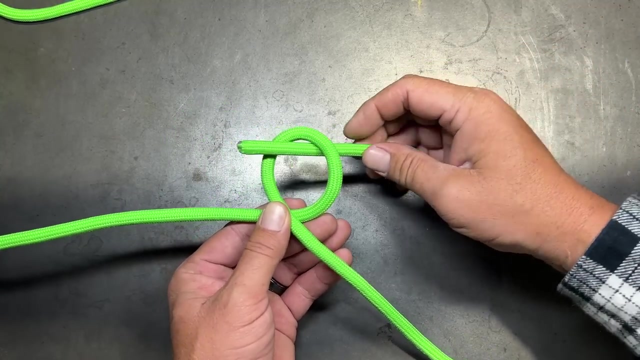 how big you want your final loop to be, And then I'm going to kind of turn my wrist over, grab the line, and then I'm going to just turn it like you would turn the ignition on your car, And that forms that first loop. Now we'll take the working end and we'll go up through that loop. 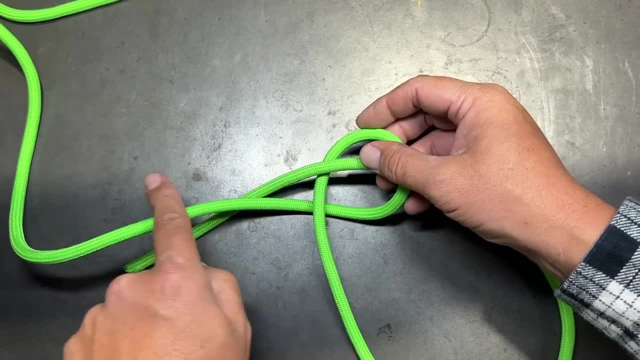 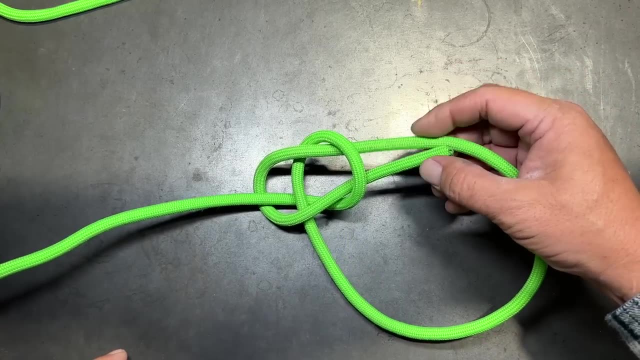 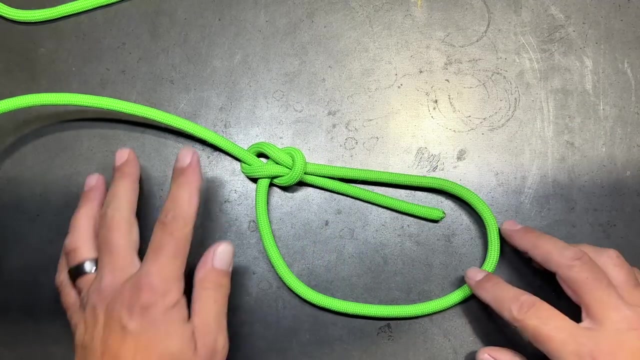 Then we'll trail it around so that it goes behind the standing end, And then we'll put it right back down through the loop that we formed. Now, at this point you'll pinch off your working end and the inside of your loop, pull on your standing end, pull them apart and that forms the bowline One. 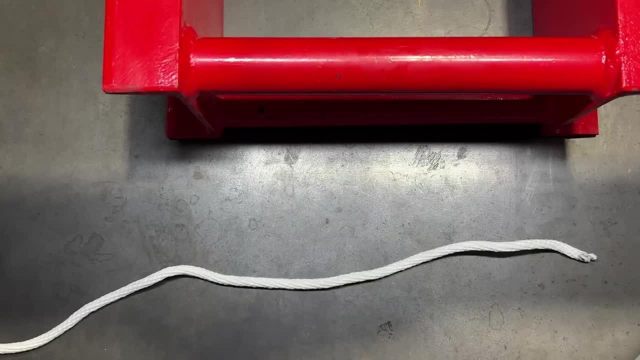 of the most important knots you could ever learn. Now, the next knot that we're going to look at is an adjustable fixed loop knot. It's called the tot line and it's also used as a friction hitch knot. You can use it to adjust the loop. It's called a tot line and it's also used as a friction hitch knot. 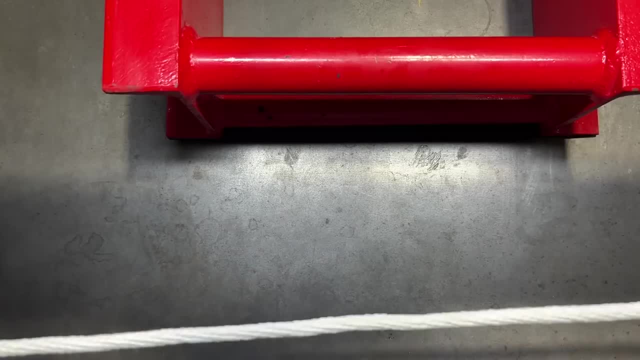 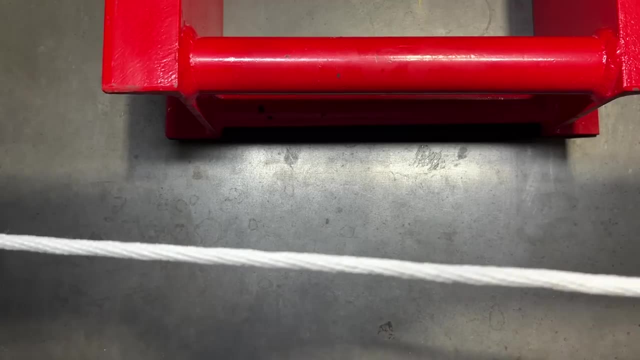 or an adjustable fixed loop knot. It's called the tot line and it's also used as a friction hitch knot, and I'll show you the difference between the two. Now I've switched ropes because with this knot it doesn't bode well to tie this with a stiffer line, So I've gone to a bit softer of a line. 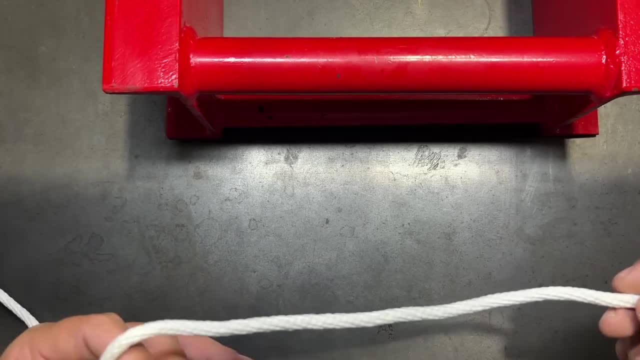 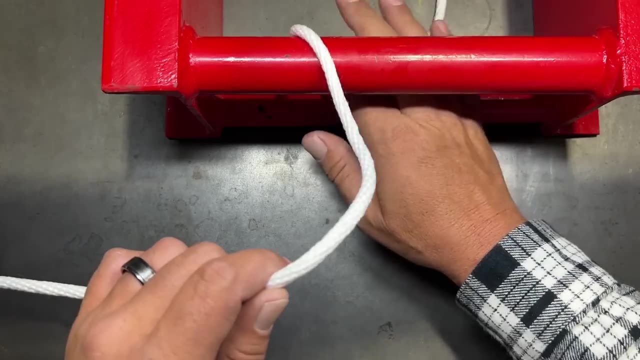 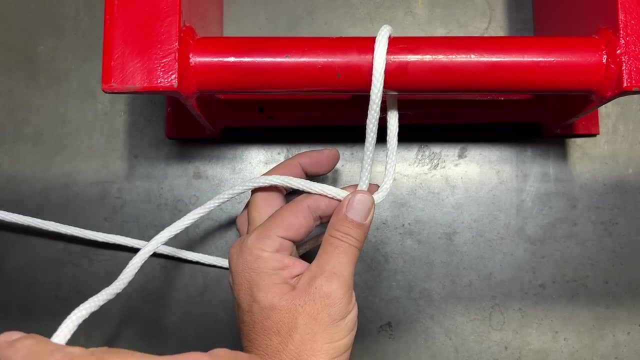 This is a good knot to use in paracord for making an adjustable fixed loop for tying, like tent stakes for tying a tent up to tent stakes. So to tie this we want to start by going around our object. I'm going to get myself a little bit more line here. Now we can cross over our standing end and 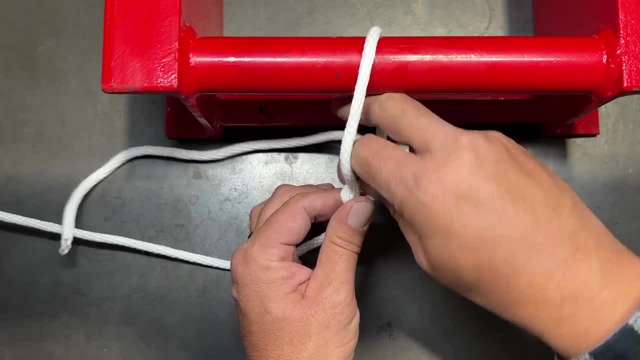 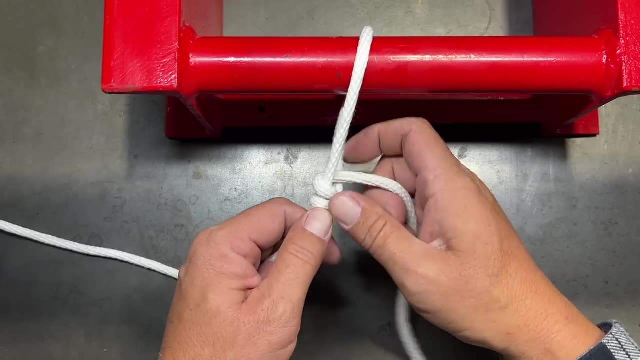 what we want to do is we want to create two wraps around our standing end, going back towards our object. So there's one and we'll go around again, and there's a second one. Now let me snug this up just a little bit, so it's a little better in view. Now, at this point, we want to just bring our tag. 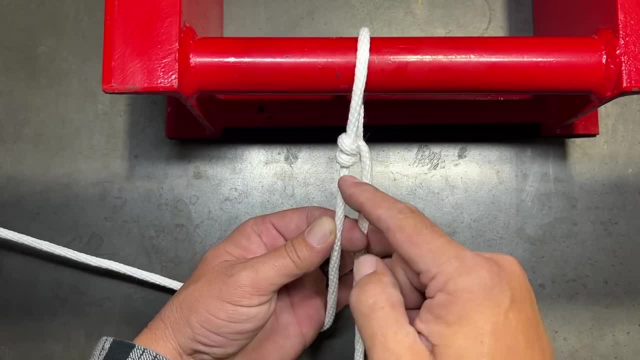 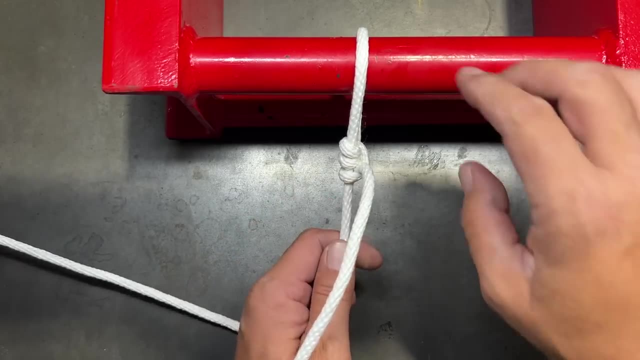 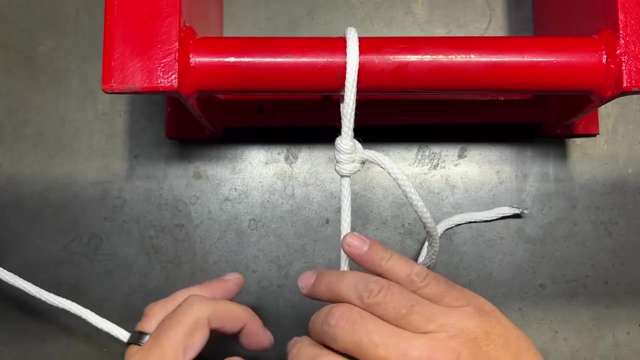 end down and we're going to create one more half hitch, but on the bottom of these two that we just formed. So if we go around the bottom, create one more half hitch going in the same direction. Now we have finished off and created the taut line hitch. Now the beauty of the taut line hitch is that, again, it's an adjustable fixed loop. 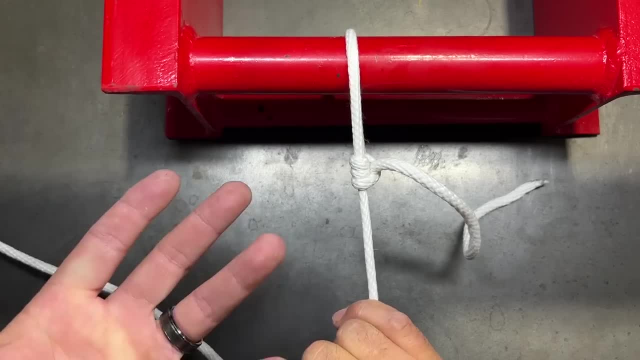 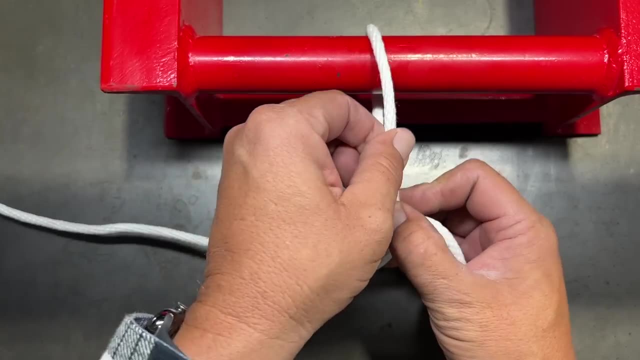 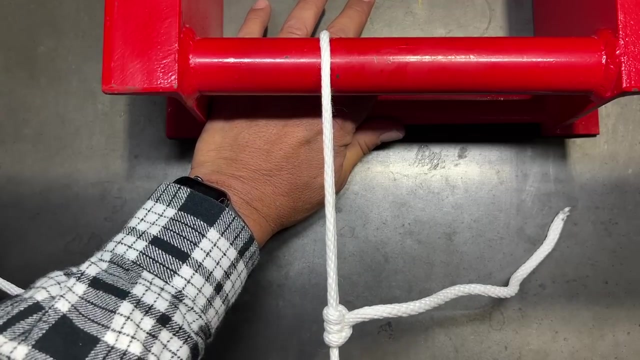 knot. So if I put pressure on this you'll notice that all those coils tighten down and keep the loop from collapsing. But because it is a friction hitch, you can easily slide this to open up your loop size or to close it down and again when you pull on it it will lock itself in place on.